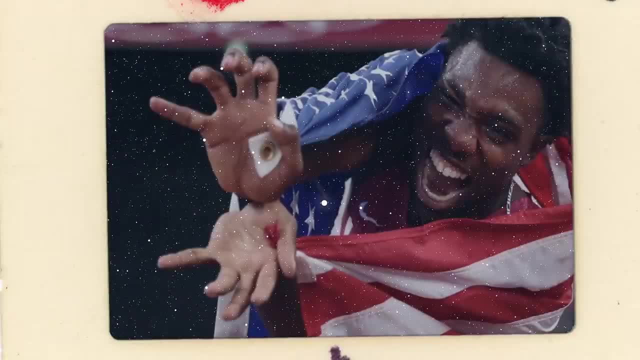 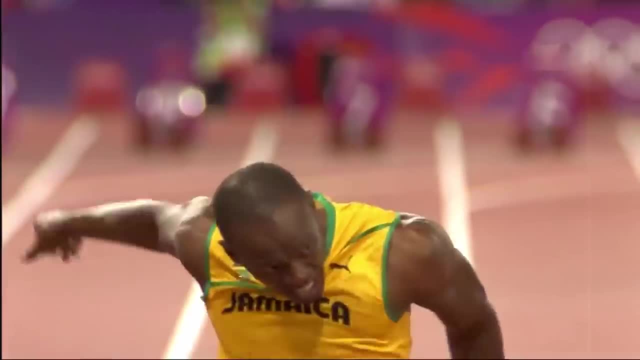 These four things are scientifically shown to make you faster. The fastest humans in the world already do them, and if we copy them, we can do the same. We're privileged to see this man in action. This is legendary pro bodybuilder, Kevin Lebron. In 2002, he challenged Maurice Green to a race. 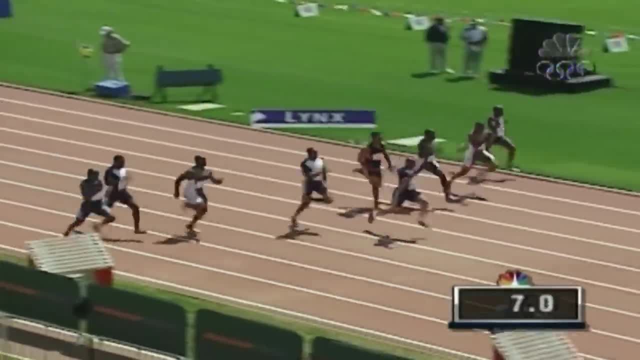 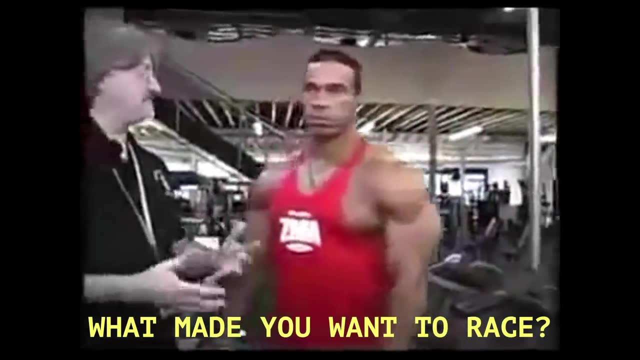 who, at the time, was the fastest man in the world. Now, what would a pro bodybuilder, now IFBB hall of famer, challenge a world champion sprinter? Tell me why. why are you doing this? What made you want to race? I'm good at running and today I'm just going to show the world you know. 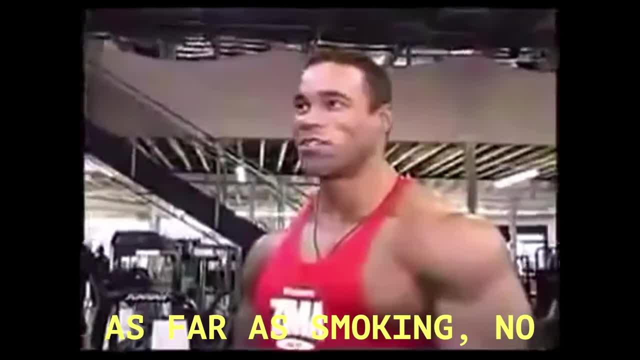 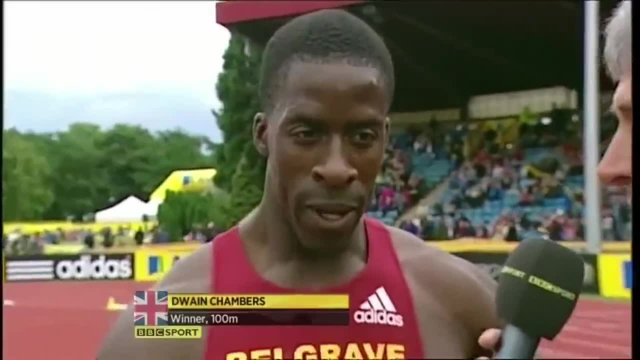 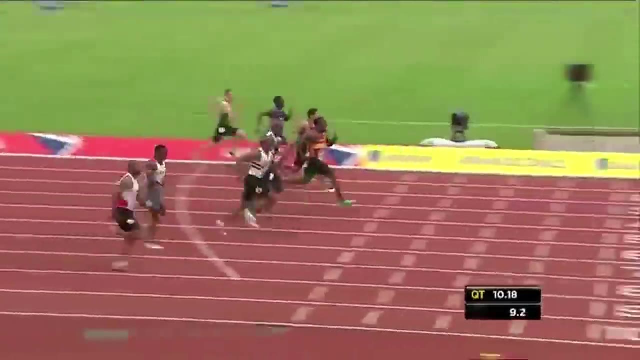 what I mean. You're going to smoke What I got, babe. Far as smoking Either way, Maurice Green never took him up on that offer, but someone else did: Dwayne Chambers, One of the fastest European sprinters in history. To this day he holds the fastest 60 meters in Europe In 2002. 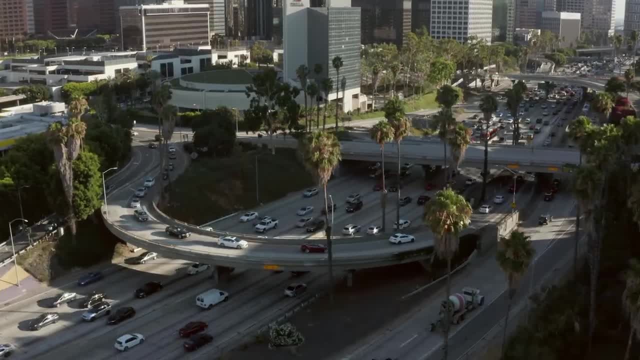 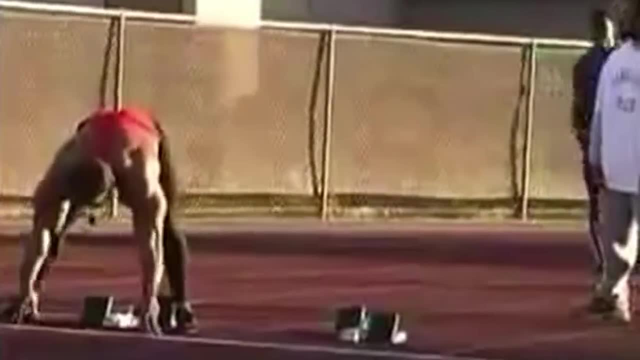 both of these guys were in the prime. The race took place in California on December 11, 2002.. It was a 60 meters race and, surprisingly, they even used starting blocks, Which, let's be honest, that alone is impressive. I mean, would you ever imagine a guy that looks like this? 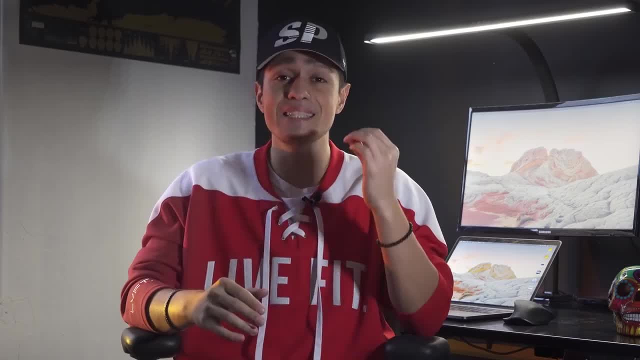 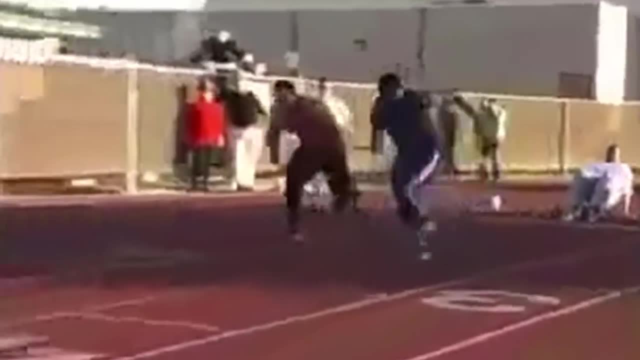 to voluntarily get into starting blocks, Much less against a champion sprinter. It's definitely not something you see every day. In terms of the race itself, well, Kevin had an explosive start, stumbled, and then it played out exactly how you would imagine. 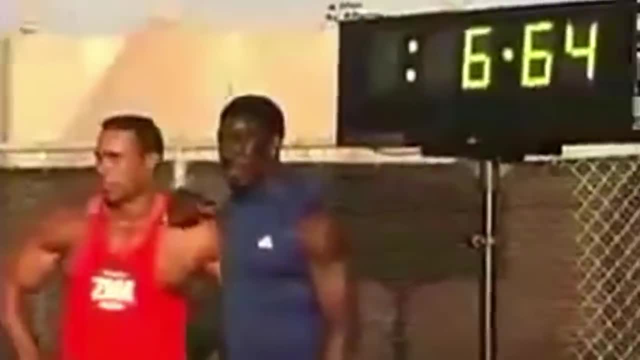 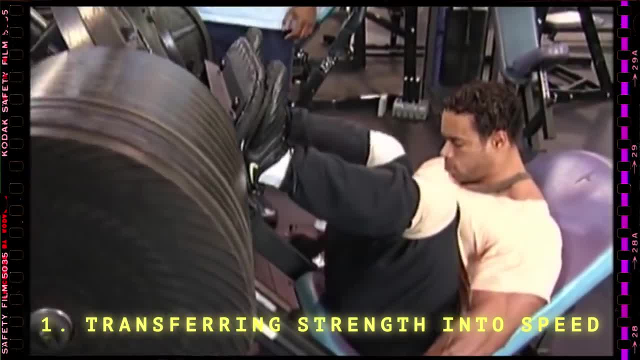 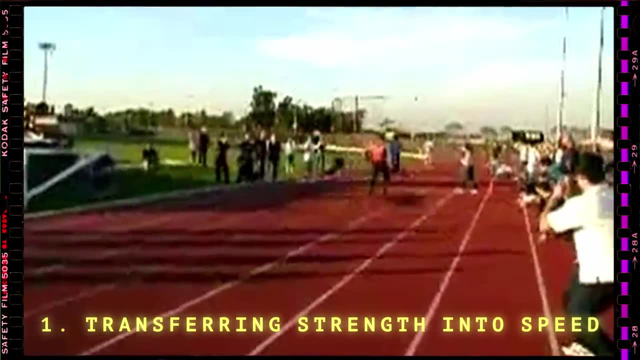 into speed. It's safe to say, Kevin Lebron had plenty of strength and it did help him produce an explosive start, Although obviously his training and physique is not optimized for speed. the fastest humans in the world may not be the strongest, but they are very effective at 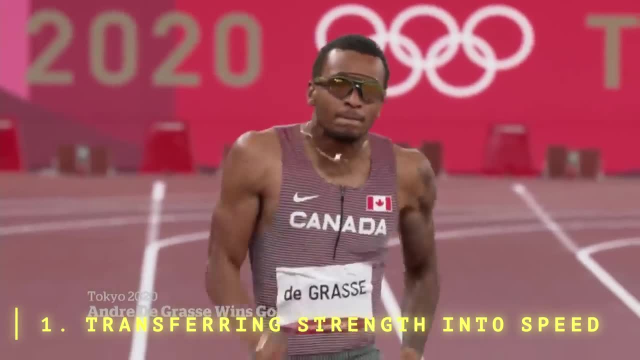 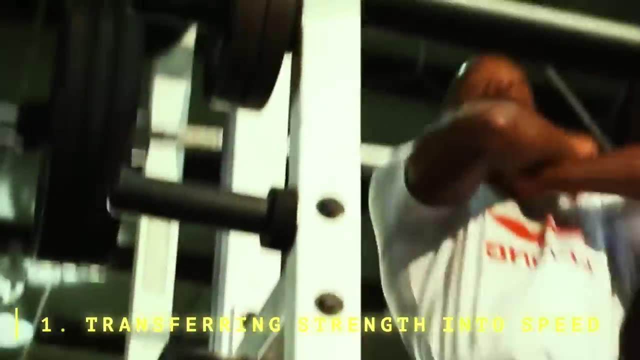 transferring their strength into speed. This is because of how they use their strength. A good example of this is Asafa Powell. Not only is he strong, he's also insanely fast. Many would argue that he has one of the most powerful starts in the history of athletics. The reason he is very 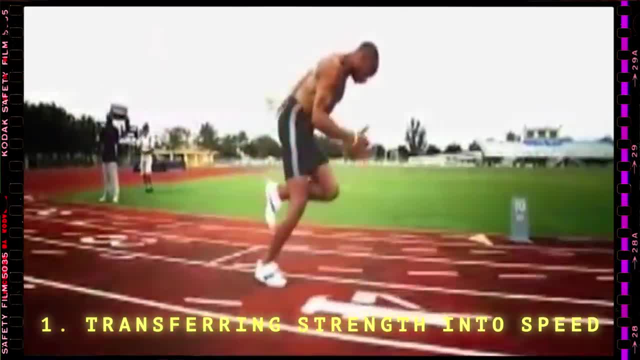 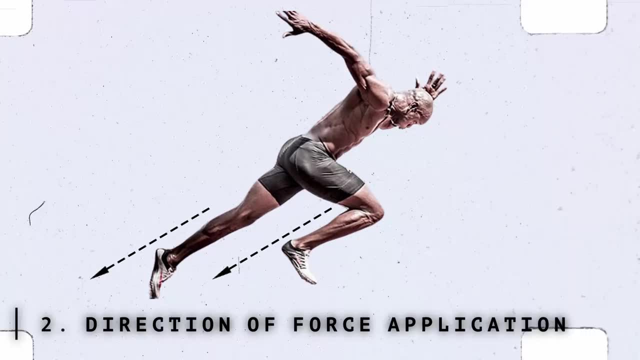 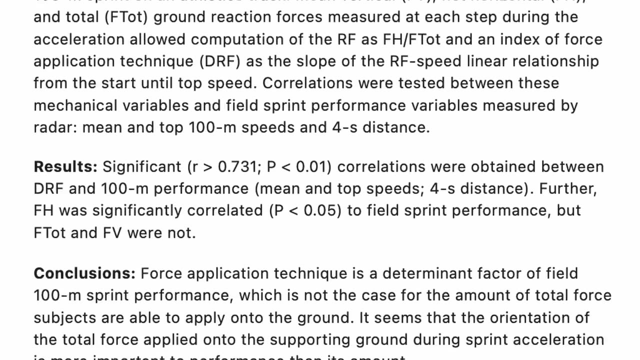 effective at converting his strength into speed is because of the direction of force application, Simply put, in the acceleration. he is a master of applying horizontal forces, which has been shown in numerous studies to lead to better acceleration times. In fact, this study even states that how. 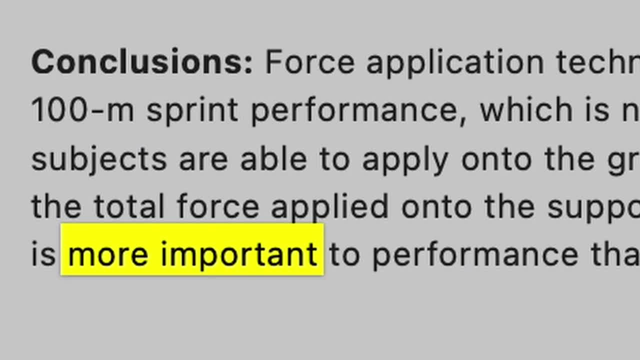 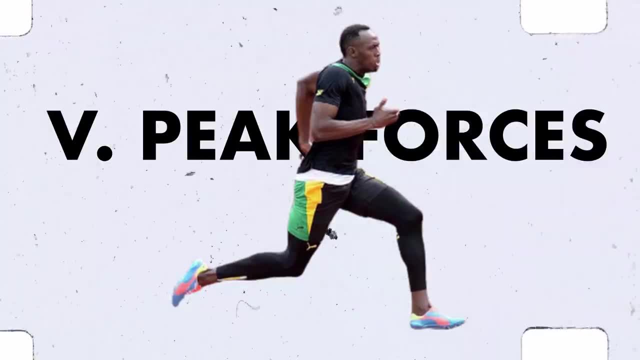 forces are applied is even more important than how much. Speaking of very strong, one of the strongest sprinters is none other than Kevin Lebron. He has a very strong body, but he has a Usain Bolt. He is reportedly able to apply vertical peak forces of up to five times his 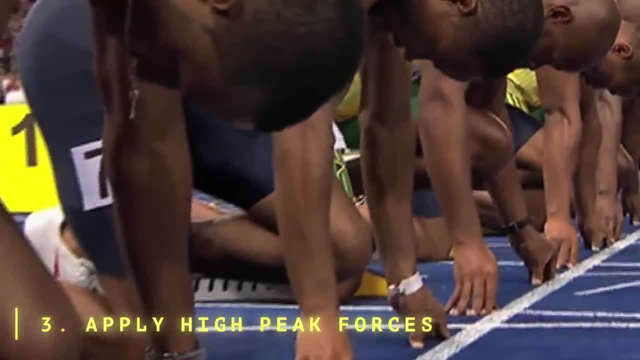 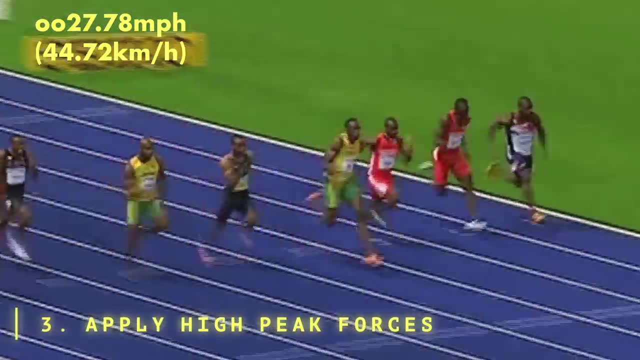 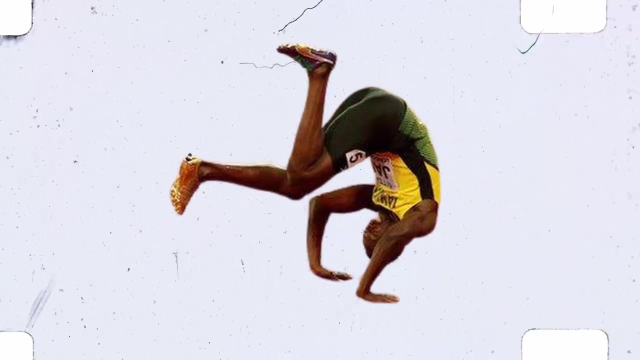 body weight. This is another thing that all the fastest humans do apply high peak forces. This allowed Usain Bolt to reach peak speeds of 27.78 miles per hour when he set the 100 meter world record in 2009.. Because he was able to reach such high peak speeds, he could fumble a start and still. 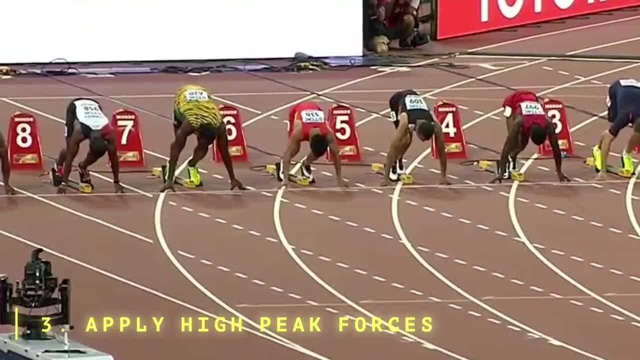 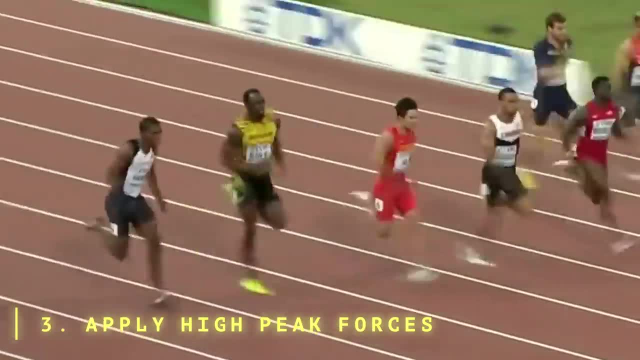 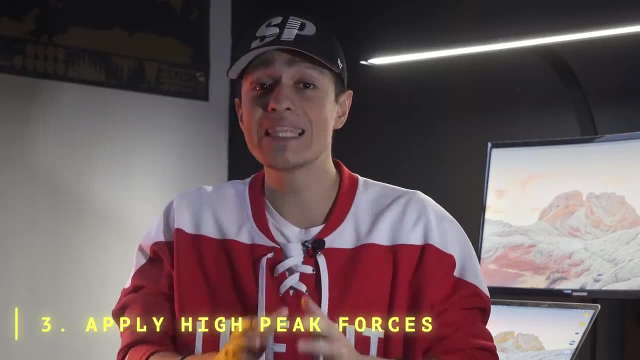 win, which is exactly what he did in 2015.. Usain Bolt stumbled out of the block and he was able to win the race in the end. This shouldn't be possible. One of the reasons he's able to do this is because of his top speed. Another reason is because how insanely effective he is at 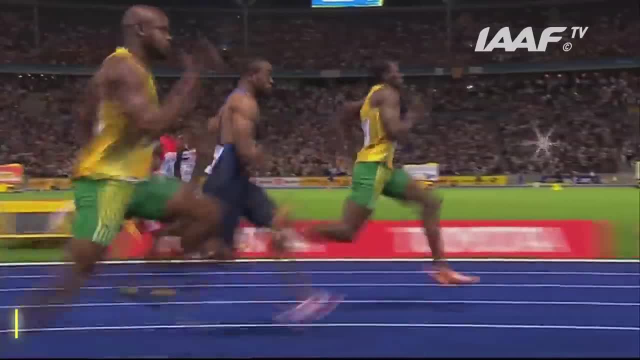 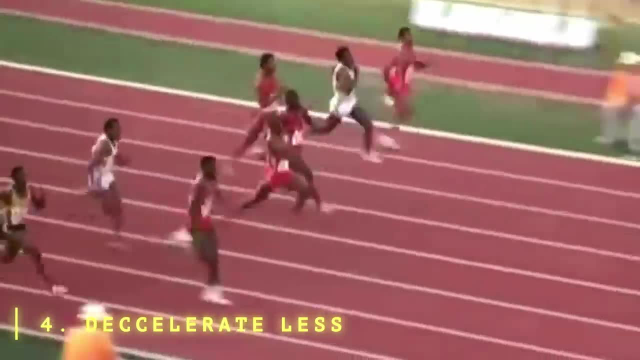 maintaining that speed, which leads us to the fourth factor: the ability to decelerate less than everyone else. As you may or may not already know, towards the end of a race, it appears as though the person in the lead is increasing their speed more than everyone. 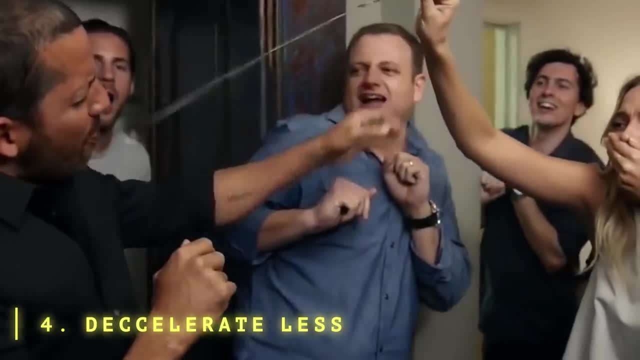 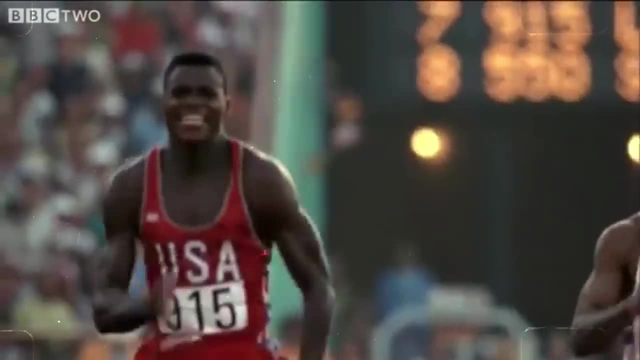 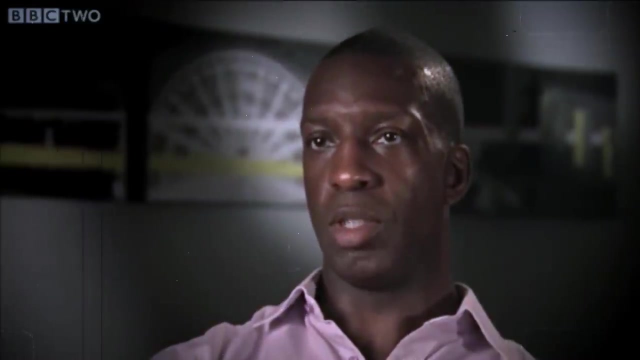 however, this is just an illusion. In reality, everyone is slowing down. It's just the winner decelerates less than everyone else. The reason Carl Lewis came first was that he could almost defy the law of sprinting. It was his signature quality that Carl would decelerate at a much. 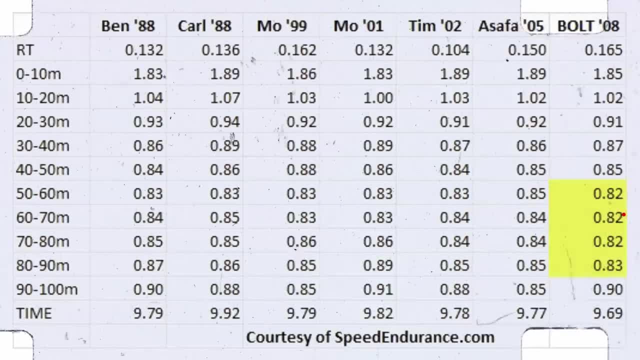 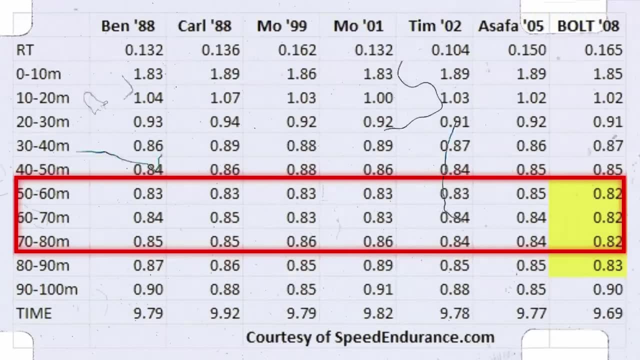 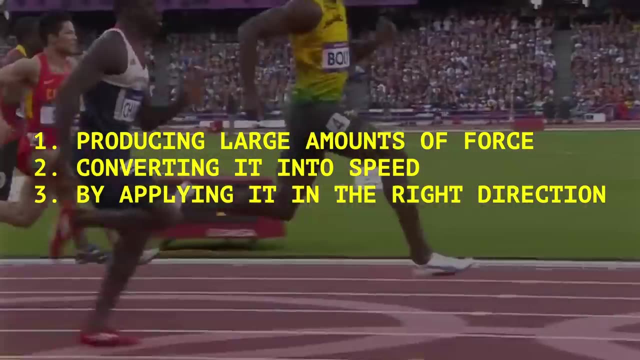 slower rate than everyone else. For example, this data shows that in 2008,, during the 100 meter world record, Usain Bolt hit his top speed and held it for 30 meters. In other words, producing large force, converting it into speed by applying those forces in the right direction and decelerating. 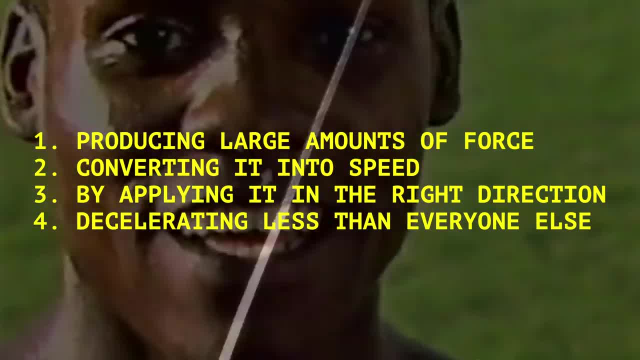 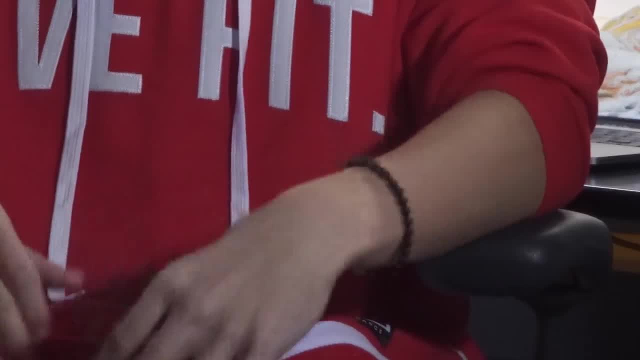 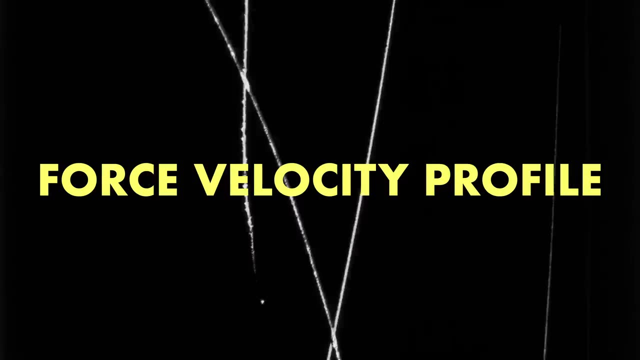 less than everyone else are four things that will lead to faster times. All right, I hope you're still following, because here is where it gets even better. I'm going to show you how you can figure out how effective you are at each of these factors through a scientific method called the. 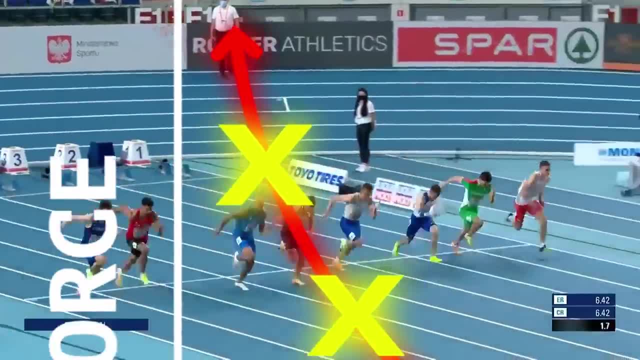 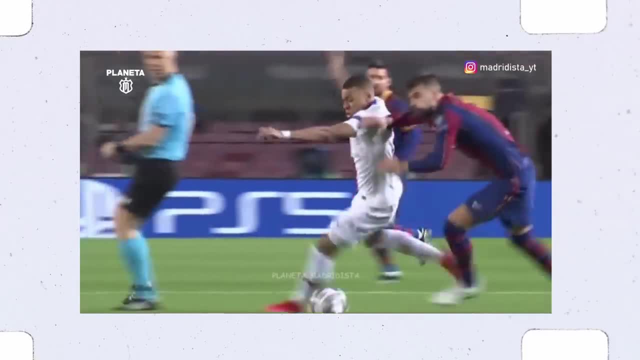 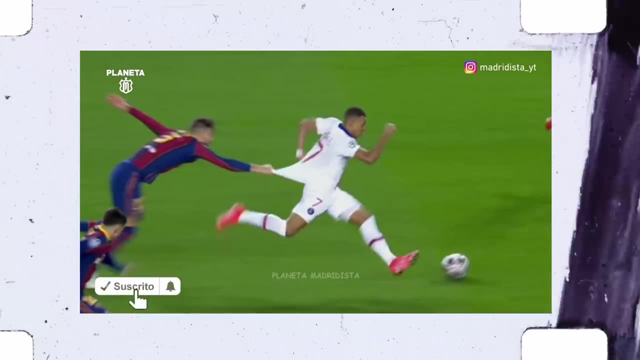 force velocity profile. If you watched my last video about the force velocity curve, then you already know what I'm talking about. As promised, in this video, I'm going to make my own FVP. If you're training in any sport that requires you to run fast, such as football, baseball or rugby, this is one of the most 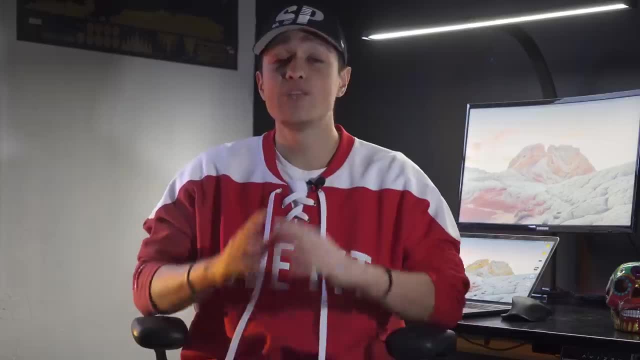 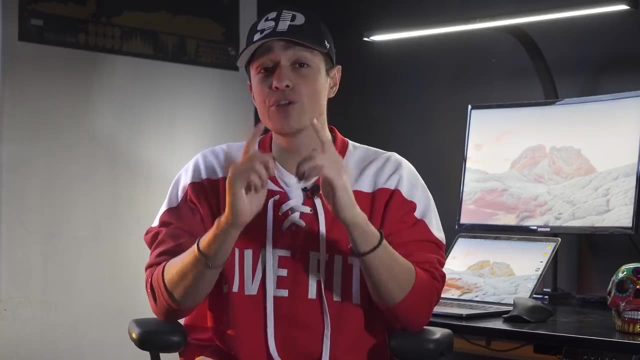 valuable things that you can do to improve your speed, And don't take my word for it. It's backed by multiple studies as a useful tool to improve sprint performance. Here is how you can do it yourself. In the last video, I mentioned that we can use the MySprint app to create our own force. 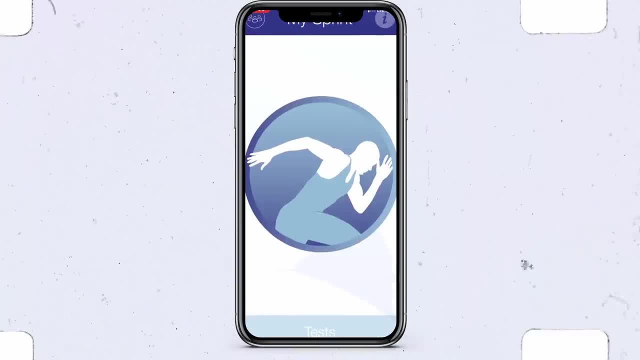 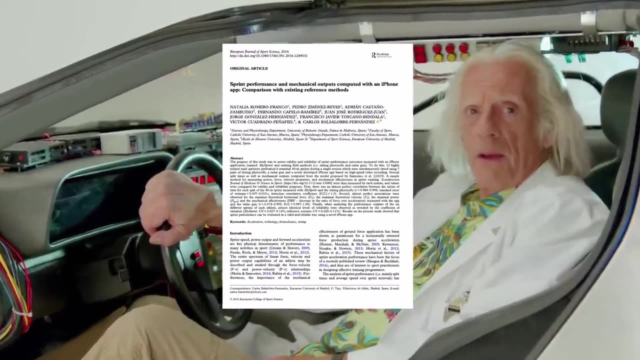 velocity profile. It's not free and, no, I don't make any money from it Currently. it's just the best option because it's backed by science as a reliable method, Although if you do want to do it yourself for free, there will be a way to do that in the 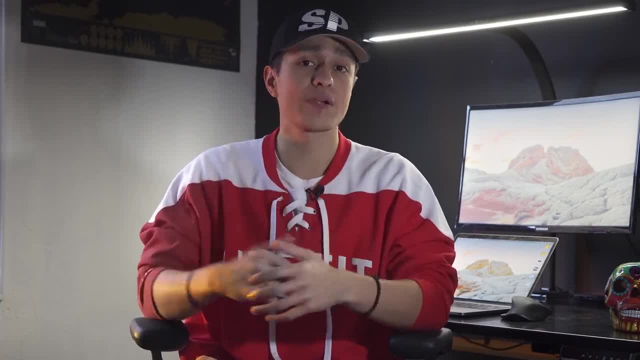 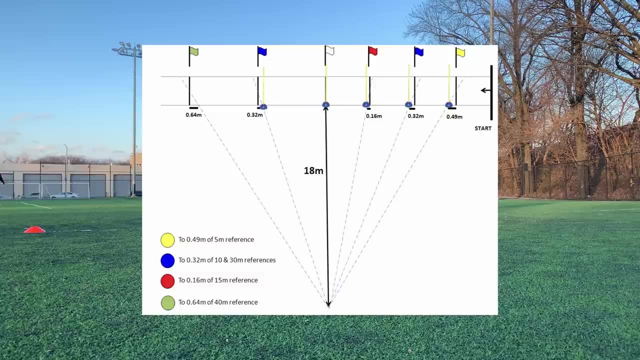 description. Just a warning: it does require a bit more work To perform the assessment. I first set up the markers, which should be placed strategically because you know when you're filming you can have a bit of distortion depending on where the subject is in the frame And, don't worry, the app will. 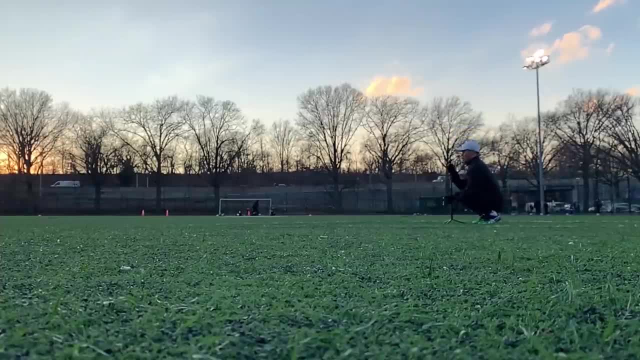 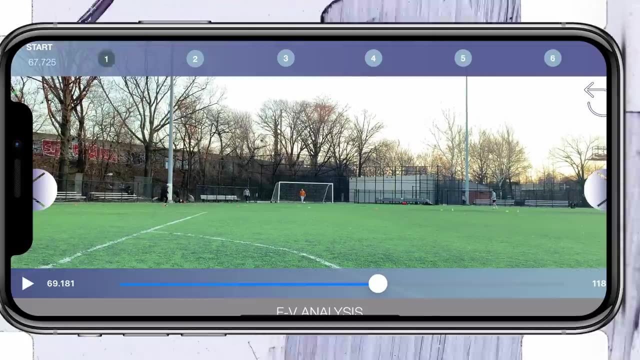 outline exactly how to do this. Second, I set up my phone on a tripod off to the side. Third, I perform the sprints. Fourth, I use the app to mark each of my splits. Finally, the app produces the calculations revealing your force velocity profile. All right, here's where it all comes. 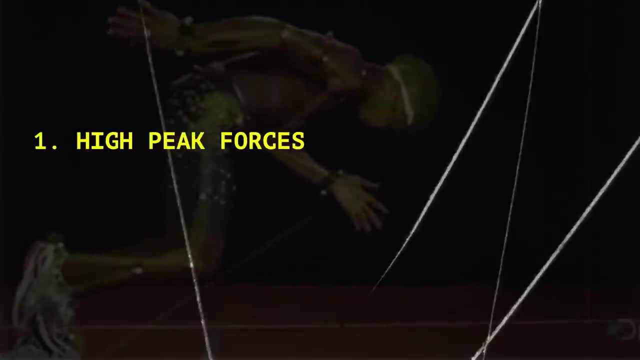 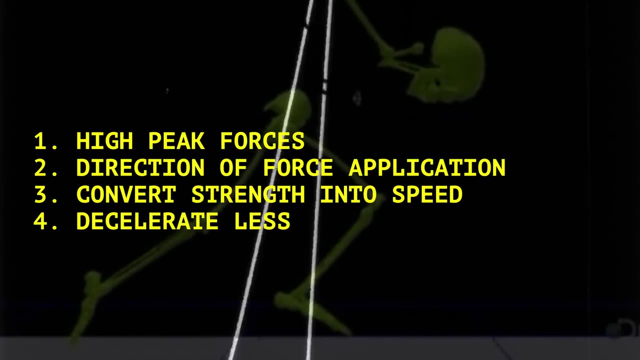 together. Remember the four things I mentioned in the beginning: high peak forces, direction of force application, ability to convert strength into speed and the ability to decelerate less Well. the numbers we see here reveal how effective we are at each of these four factors Once you. 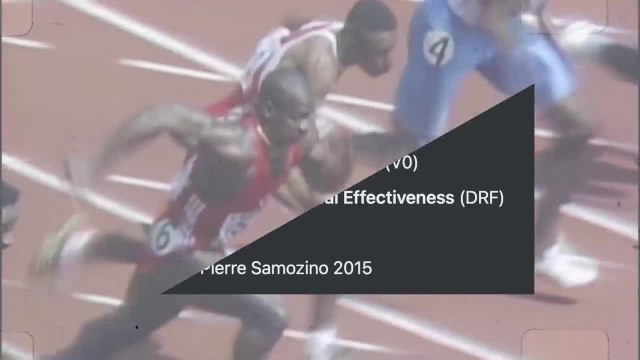 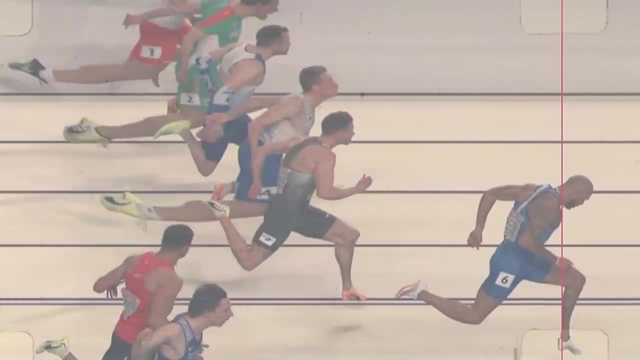 have this data yourself, you will also know what you have to focus on in your training. If you would like me to make another video in this series that goes over the science of how to target each of these factors, let me know in the comments. For now, if you'd like more information, you can go.